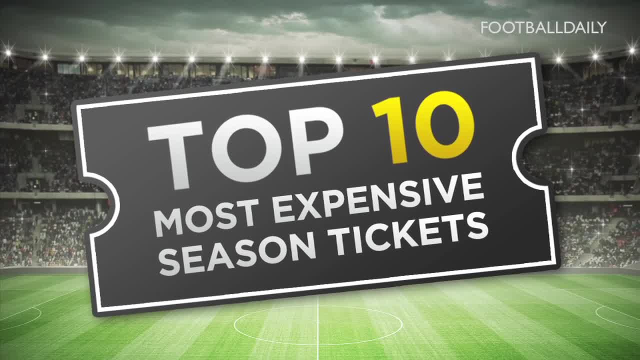 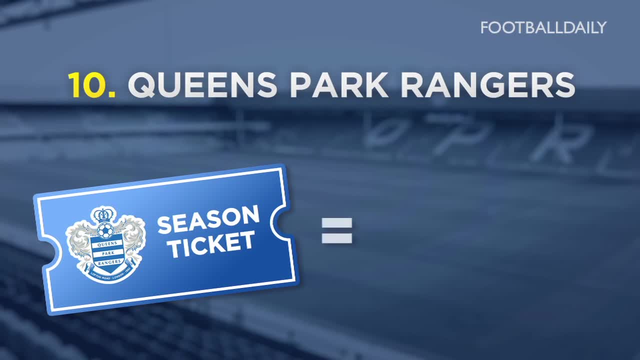 You're watching Football Daily. This is the top 10 most expensive season tickets in Europe. First up is QPR. The West London club's cheapest season tickets are still a pricey £499,, making them the 10th most expensive in Europe. Incredibly, that's more than the cheapest season. 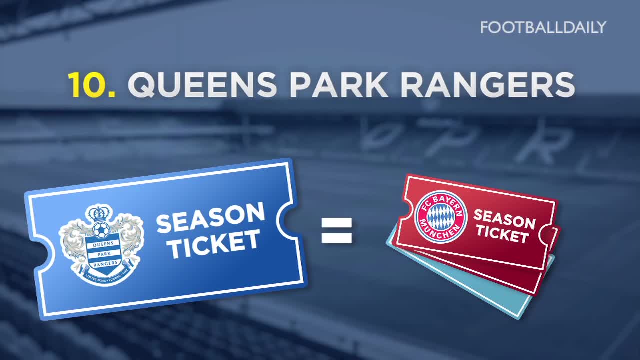 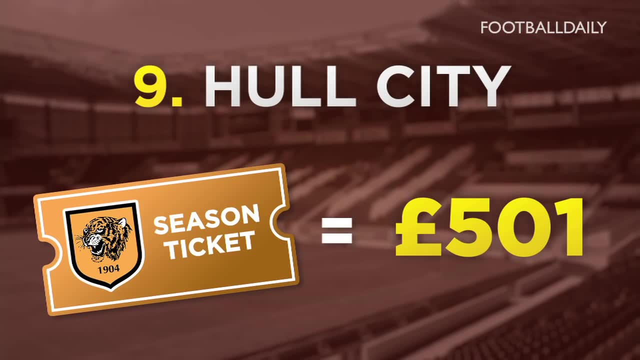 tickets on offer at Manchester City, Atletico Madrid, Bayern Munich, Juventus and PSG. At nine is Hull City, with the Tigers' most reasonable season tickets on offer, at £501.. Ahead of Hull is Newcastle United, Despite having the cheapest available matchday tickets. 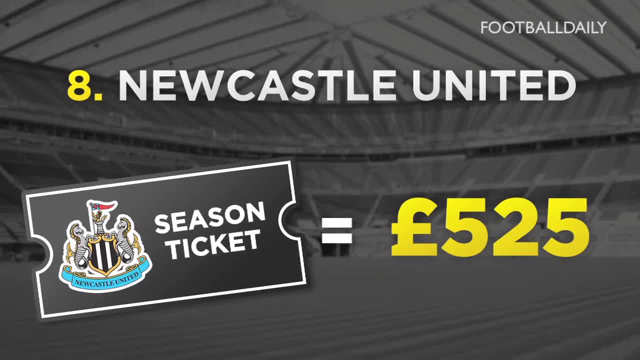 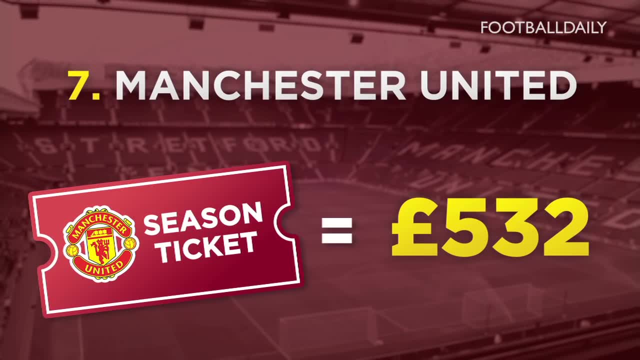 in the Premier League. Newcastle's cheapest season tickets are still the eighth most expensive in Europe. At seven is Manchester United. The Red Devils' most reasonable season ticket is available for £532,, more than five times the price of the cheapest at Barcelona. Sixth is Southampton Not. 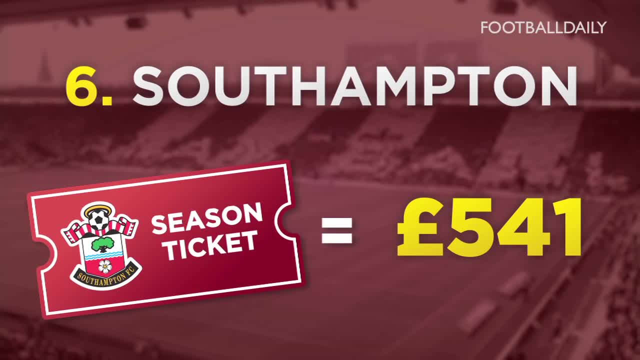 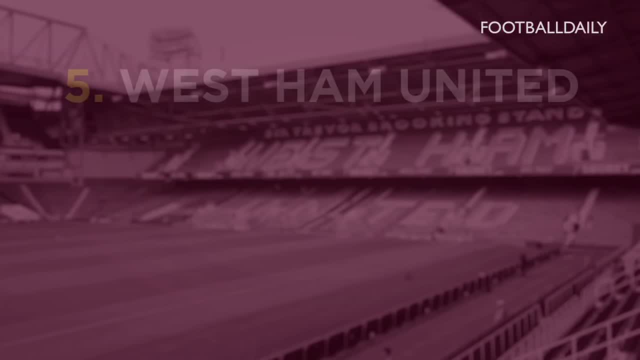 only are the Saints' cheapest season tickets, the sixth most expensive in Europe, they also charge more than any other Premier League club for a programme, a pie and a cup of tea At five is West Ham United with £670, the best offer for season tickets at Upton Park. 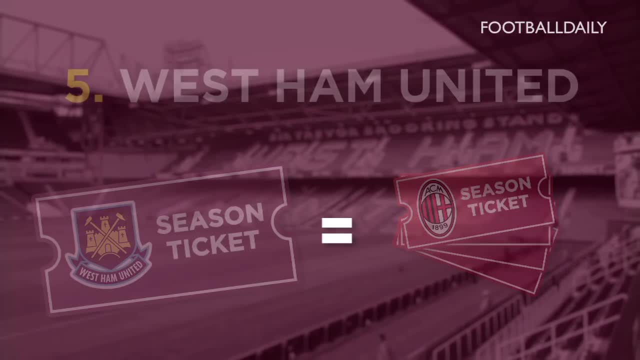 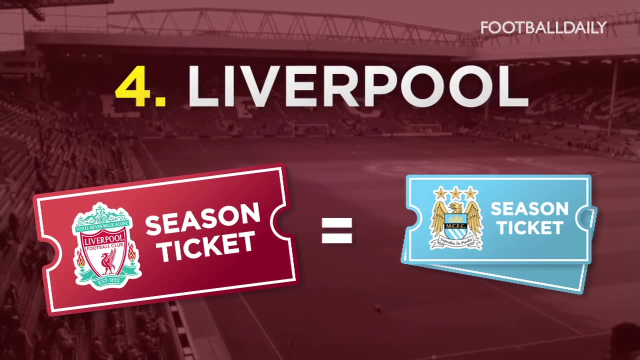 over four times the cost of the cheapest available at AC Milan. Number four is Liverpool. At Anfield, the cheapest season ticket will set you back over £700, more than double the cheapest available at Manchester City. In third place is Chelsea. The Blues' cheapest available season ticket is £750. 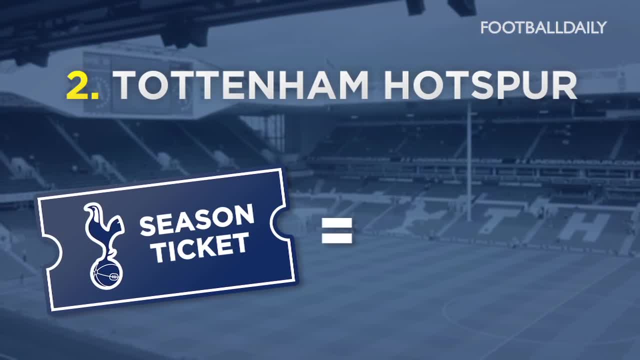 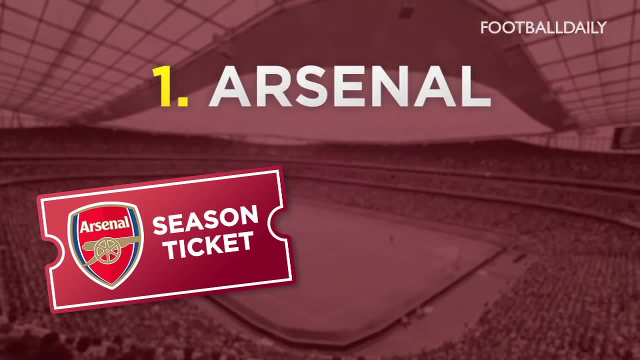 In second place is Tottenham Hotspur. The North London club's cheapest season ticket costs a hefty £765, the most expensive in Europe, second only to Arsenal with the cheapest season ticket on offer at the Emirates, a whopping £1,014.. For the same amount, you could buy four. 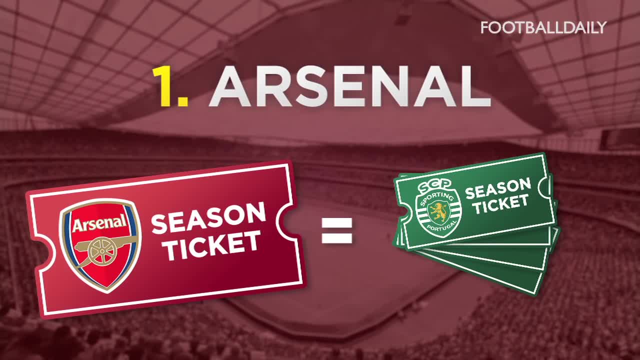 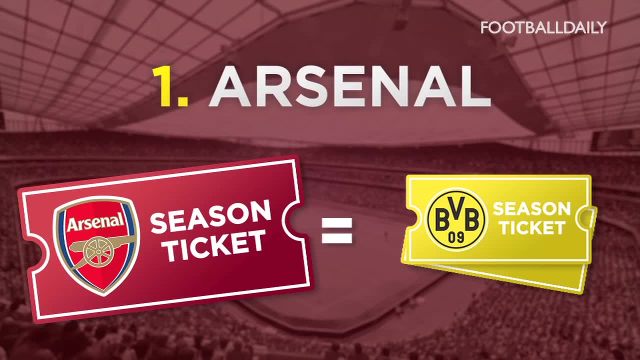 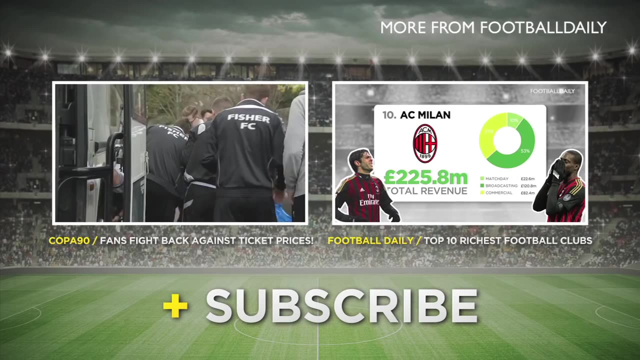 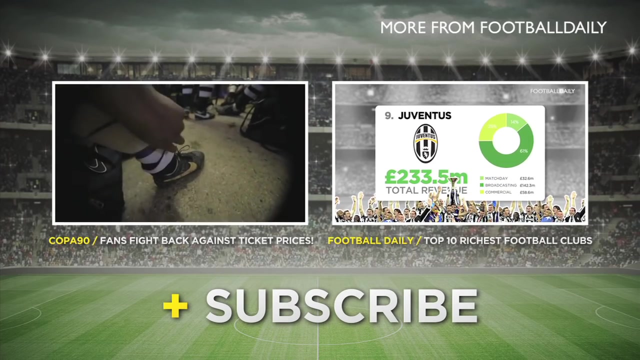 of the most expensive season tickets available at Sporting Lisbon and still have £13.40 left over. For the same price, you could even nearly afford two of the most expensive season tickets at Borussia Dortmund, A fantastic non-league club with a fantastic set of supporters. 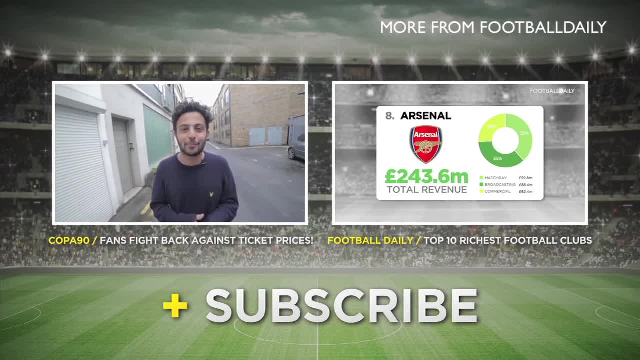 who helped save the team that they love and are trying to get them home to Bermondsey.